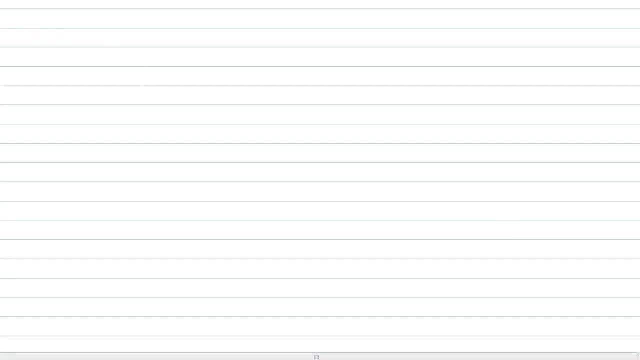 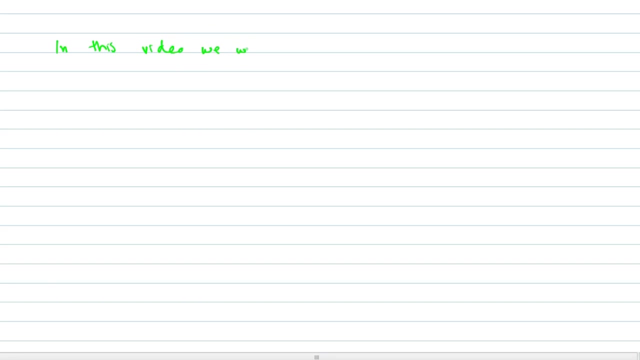 Welcome, friends, Welcome to step-by-step tutorials. In this video we will learn that what is a crystal lattice? what is a unit cell for a lattice, what are brevis lattices and, finally, what are bases for a crystal structure? An arrangement of infinite number of points in three-dimensional. 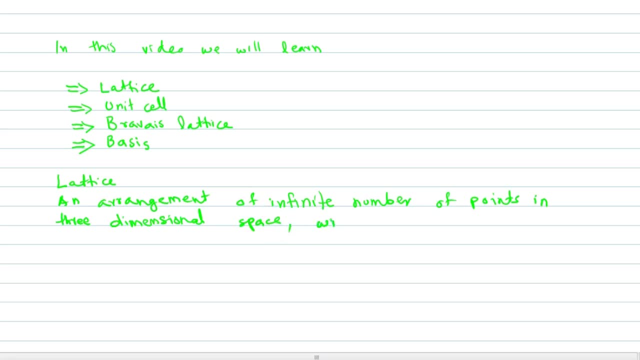 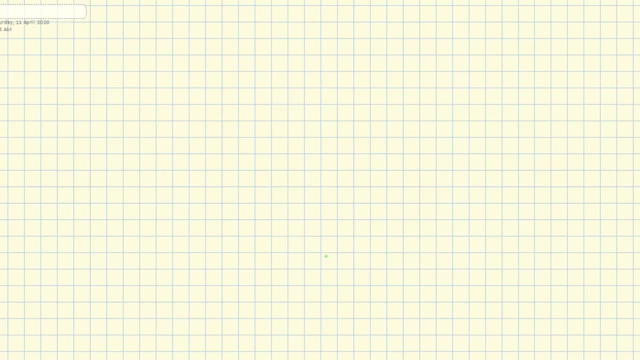 space, with each point having identical surrounding is known as lattice For the lattice. the most important point is that each point having identical surrounding. So now we will draw a lattice structure by starting with a single point, surrounded by four other points in a some specific pattern. 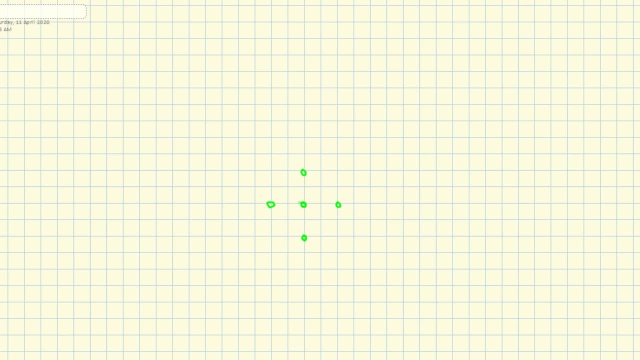 As you can see that the one point is surrounded by four others. Now, what we will do? that we will give identical surrounding to all points. So I am drawing another points such that all points get identical surrounding. As you can see that, as I continue this process, 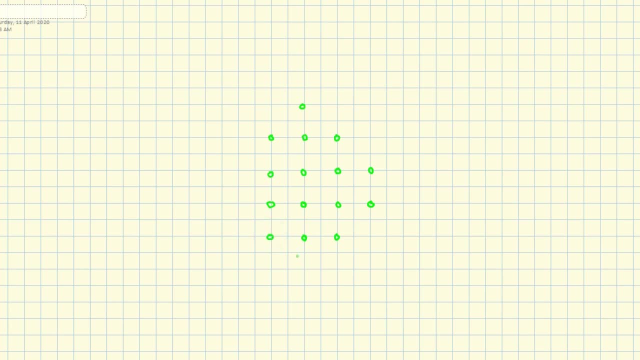 So you can see that a proper pattern is being generated. So my primary aim was only to give identical surrounding to all points. So, as you can see, the pattern with boxes- square boxes- Is being generated. So I will continue this process up to certain limit. 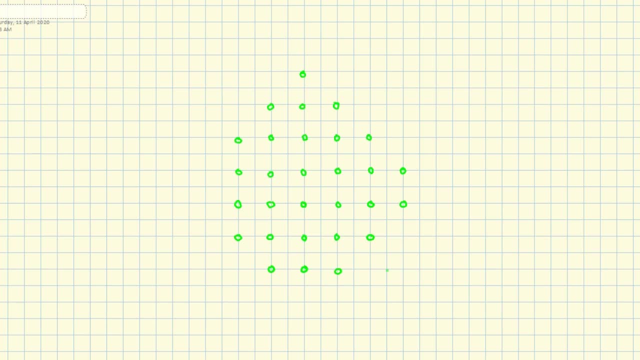 So that pattern becomes visible By now. I think that this pattern will be visible for everyone, But anyhow, I will come And complete this pattern So as we can see that proper pattern is being generated, Although I was only trying to give identical surrounding to each and every point. 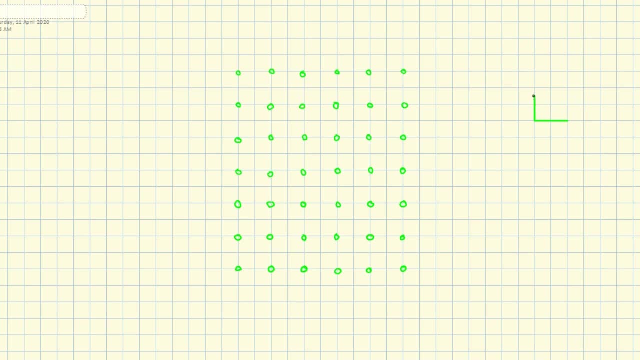 And automatically a pattern is being generated. So, if this is your y axis And this is your z axis, So now you will see that there is a proper square shaped pattern everywhere, Whether you move along y axis or along z axis, In which ever direction you go. 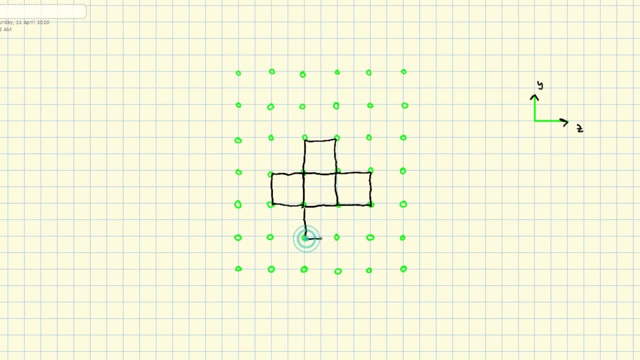 You will get this specific proper pattern. So now you will see that there is a proper square shaped pattern everywhere. So it means, if we go on extending this pattern in any direction, In all directions, So it will make a proper lattice structure. So these are the sides A and B. 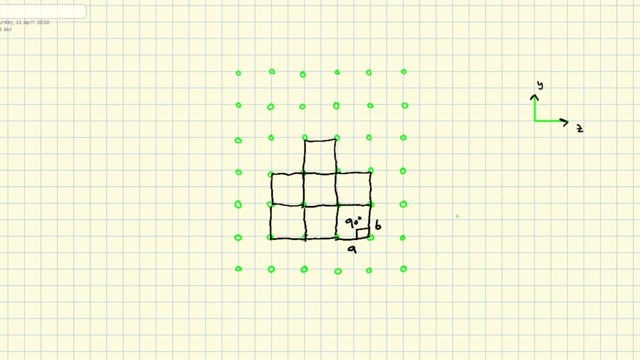 And the angle between the A and B is equal to 90 degree. So sides A and B and angle between them are called lattice parameters. So sides A and B and angle between them are called lattice parameters. So sides A and B and angle between them are called lattice parameters. 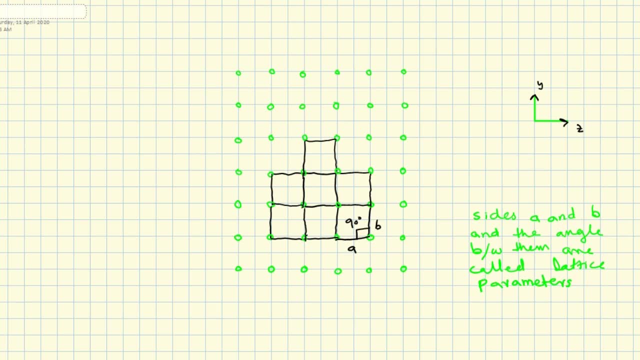 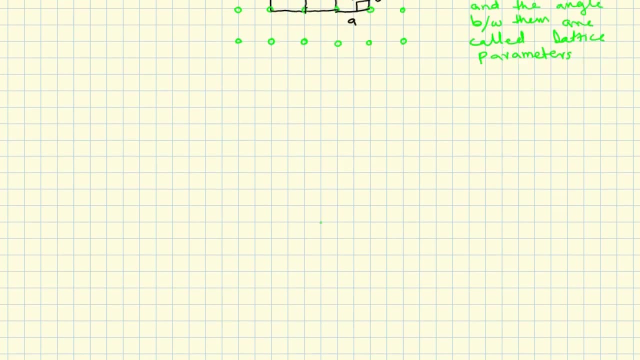 Now, once again, we will take another pattern. I will take a single point And surround it by four other points, But in different manner. So now, once again, I have taken one point And I have surrounded it by four other points. Now I will continue on. 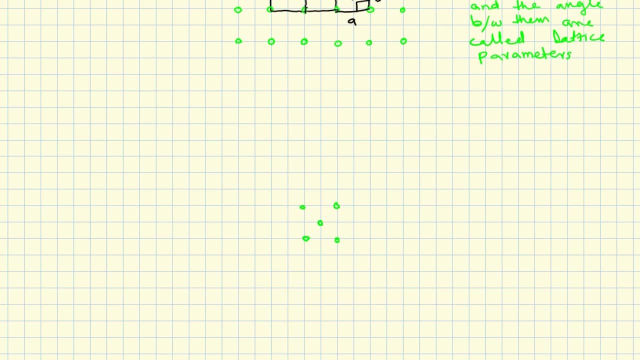 Giving the identical surrounding to the each and every point here, So I will surround this point by four other points in a similar manner. Similarly, now this point. Previously, we also surrounded one point by four others, But the pattern was different. Now, as you can see, once again a proper pattern is being generated. 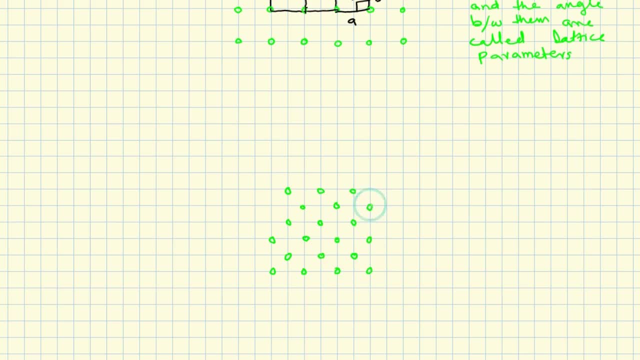 But this time the pattern is different from the previous one. So I will continue on this process until I get a very visible pattern. So this time, I will continue on this process until I get a very visible pattern. visible pattern. So, as you can see, the more I move on, the more pattern is being getting visible. 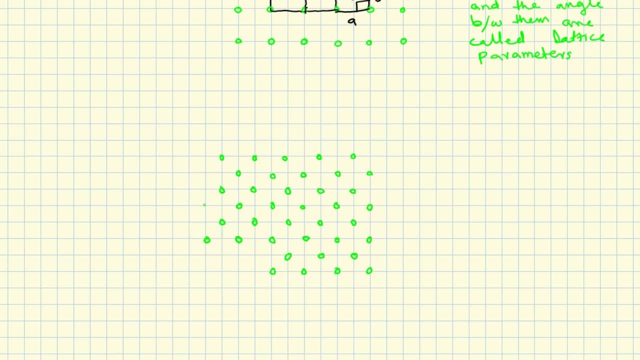 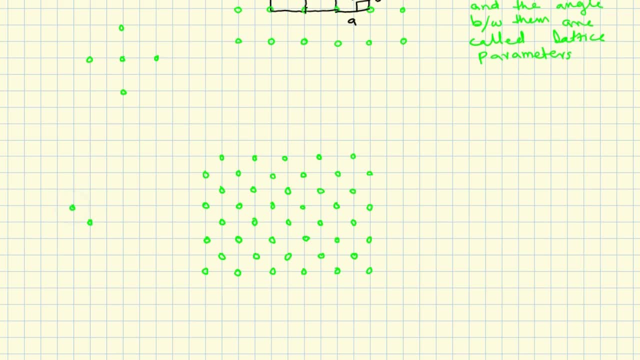 although in both the patterns i surrounded one at one point by four other, as you can see, the pattern is different. so first thing we get that, the lining of the points, as you can see. after that, the another thing we note down here is this box: in whichever direction you go, 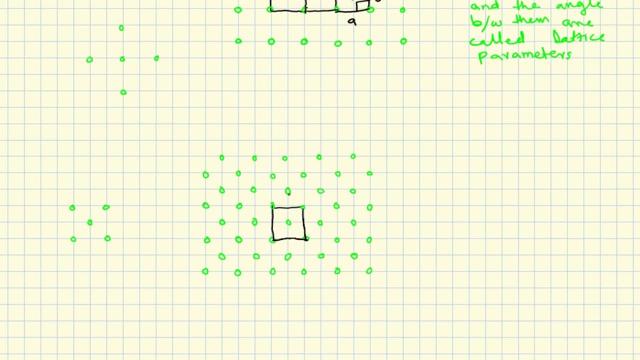 you will find this type of box, that is, a box with a central point that is just like a face centered, that at each face you have one point. so this process will continue in whichever direction you go. so, as you can see, initially our aim was only to give identical surrounding, so this specific box or square with one central point is your. 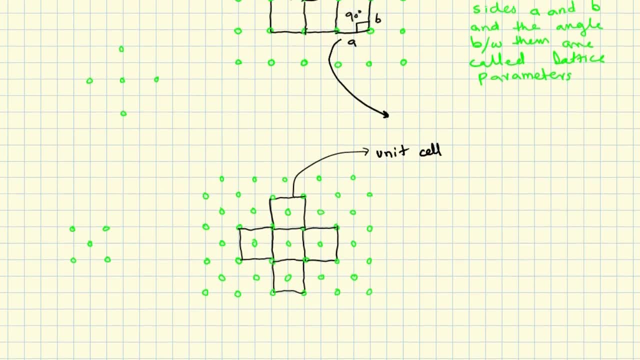 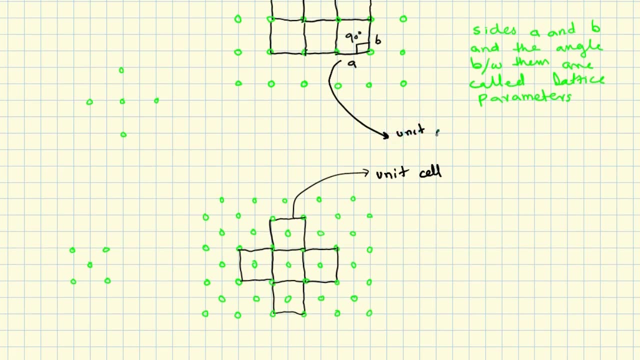 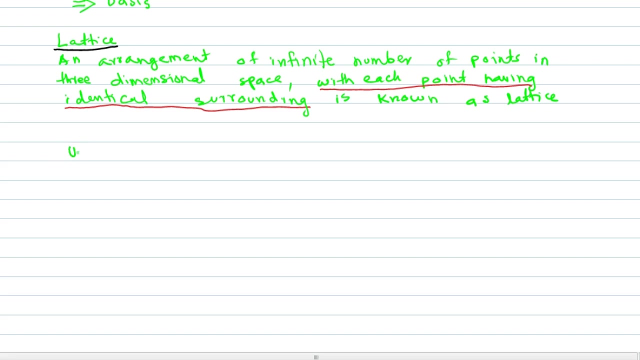 unit cell. as we can see, for the previous previous one, this unit cell was a quite different one. so this is a unit cell for the previous pattern, and this pattern is your face centered. so now we will understand what is a unit cell. we will define it so. 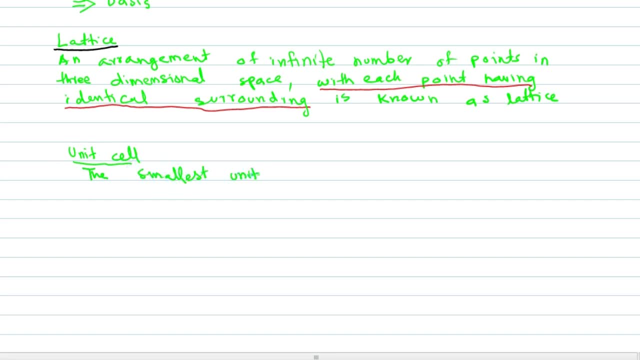 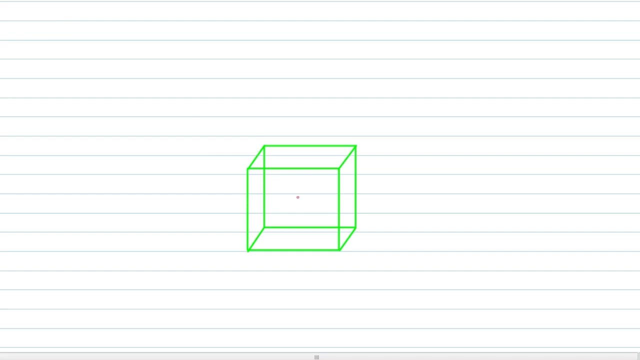 unit cell is this the smallest unit of lattice which, on periodic repetition along three dimensions, produces a complete lattice and oke, we will come back to this point in this table afin to be able to prove that this complete lattice is true. So now we will move our discussion to the three-dimension. As you can see, we have one. 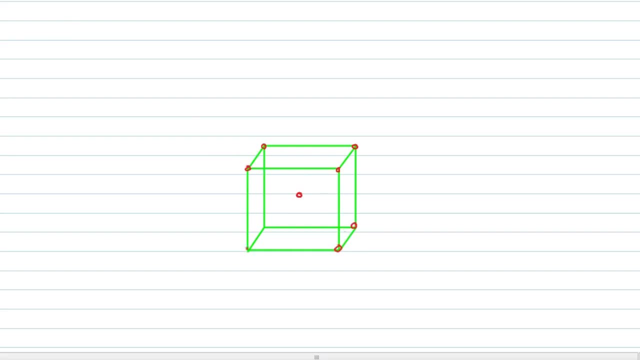 central point here that is surrounded by eight other points in a cubic manner. So we have one point surrounded by eight points in cubic symmetry, So by definition that all points will be having identical surrounding. So I find the surrounding for this specific darkened point, So to find that I have drawn seven other. 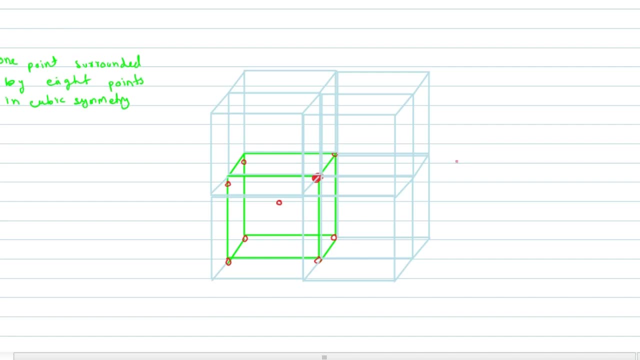 cubes along the previous one, As you can see that I have drawn the new cube with a light color so that the initial one is visible and prominent. So this is just the repetition of unit cell, But I haven't assigned the lattice points. 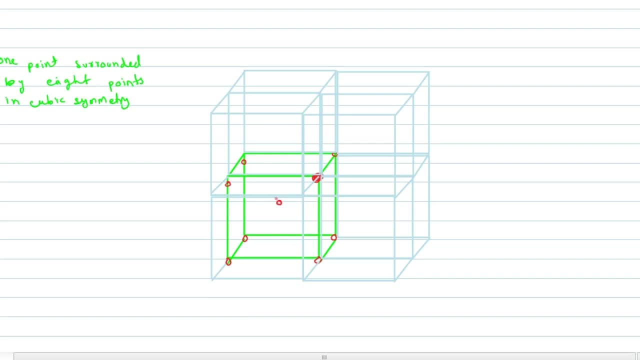 in these unit cells. yet, just to avoid confusion, So we have to find the surrounding of the darkened point, So the centers of the all cubes with one single cube, such that the centers of the cube will lie at the corners of this new cube. 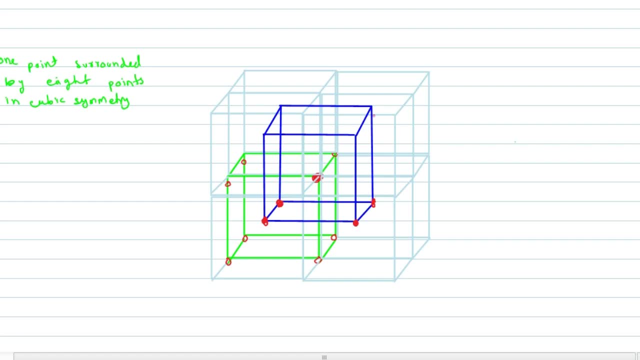 that is colored as blue. So I am pointing out the center of the all cubes, at the corner of this new blue cube. So, as you can see that these eight points have surrounded the initial darkened point, So we can see that the symmetry of all points, 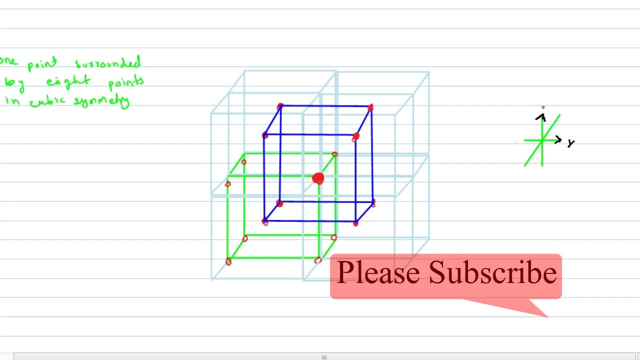 are same. All points are surrounded by eight other points. So if these are your xy and z-axis, so this will be the y-axis direction, this will be your z-axis direction and this your x-axis direction. So if we continue these cubes in all these three, 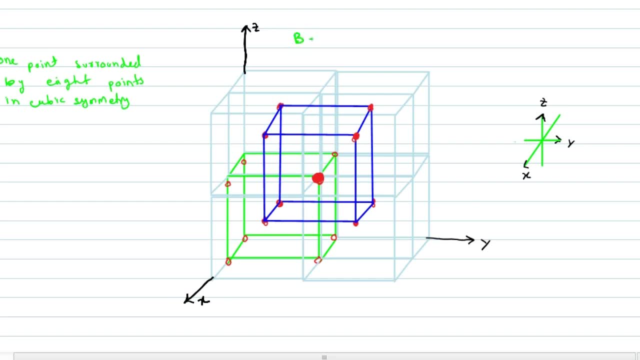 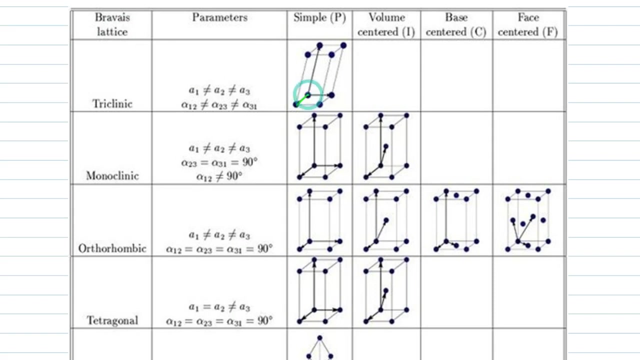 directions we will get a proper lattice structure for body centered cubic lattice. So now we come to the bravest lattices. as this topic is easy and frequently found in physics and chemistry textbooks, So we will not put much effort into this topic. So first, three parameters are a1, a2 and a3. 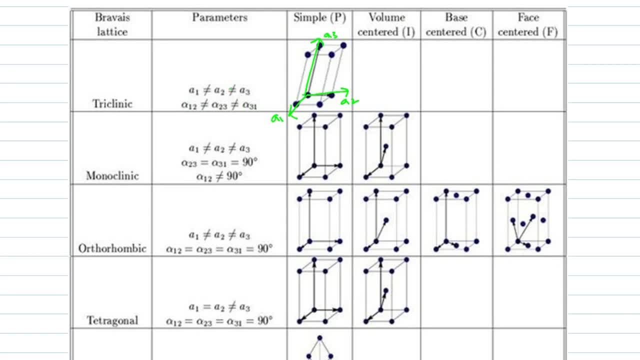 and the angle between them are alpha 1,2,, alpha 2,3 and alpha 3,1.. So for the triclinic, the a1 is not equal to a2, is not equal to a3 and all the angles are different. For monoclinic, alpha 1,2 is not. 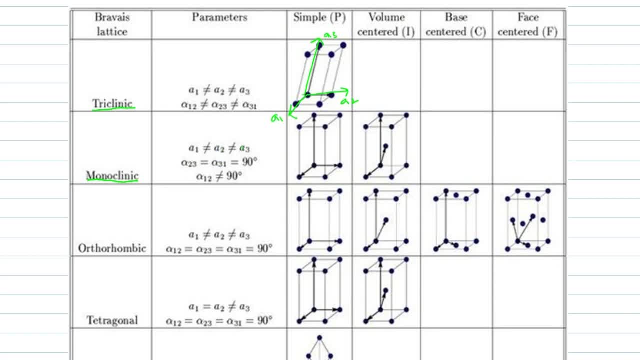 equal to 90 degree. the rest of two angles are equal to 90 degree and all the three sides are different from one another. For orthorhombic, all sides are different from one another and all angles are equal to 90 degree. 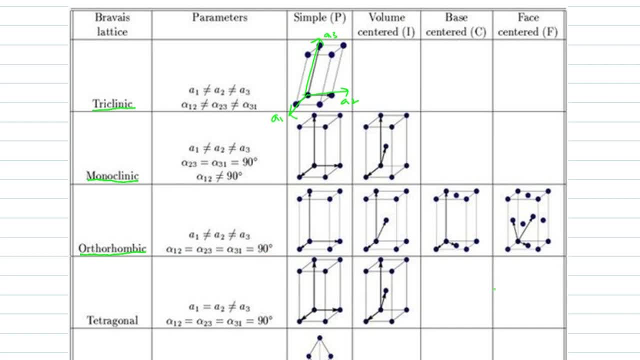 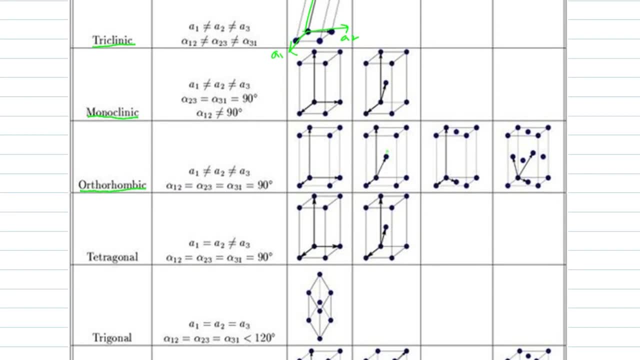 There are four formation for this specific bravest: lattices. So that is the simple one. and the volume centered, or body centered, this one. and we have end centered and finally we have face centered, That is, each face is having one lattice point. Now we have tetragonal. 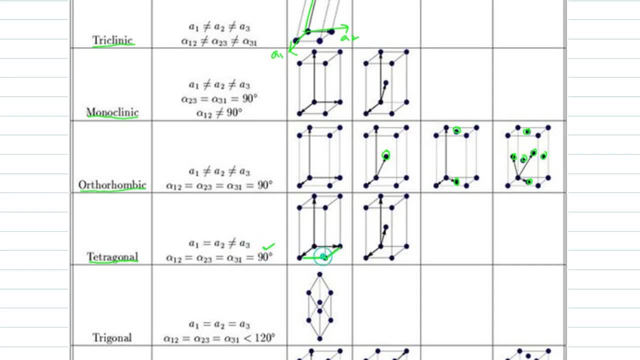 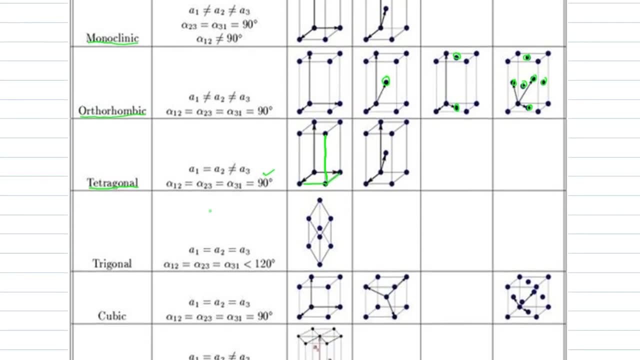 For the tetragonal we have the all angles are equal to 90 degree, but the side a1 is equal to a2, but that is not equal to a3. Means the a3 is different from the rest of two. Now for the trigonal. we can see that the side a1 is equal to a2, is equal to a3, but 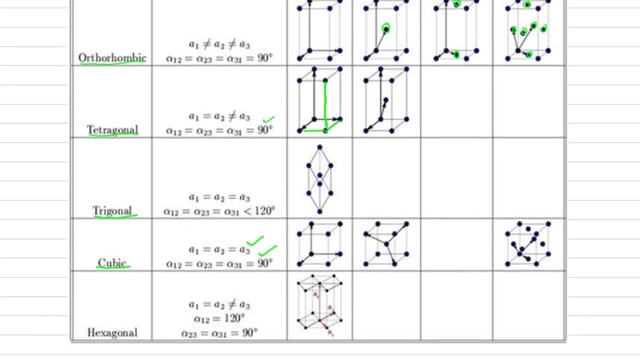 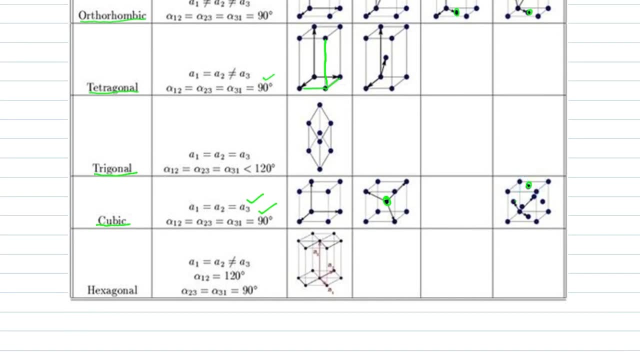 all the angles are equal, but less than 120.. For cubic one we have all the sides are equal to one another and all angles are equal to one another. It also have the three formation that are the simple body centered and face center. For the hexagonal we have decide A1 is equal to A2, but that is not equal to A3.. 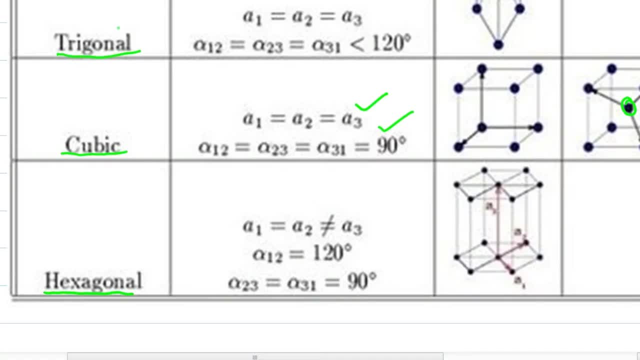 And the angle 1, 2 is equal to 120 degree and alpha 2, 3 and 3, 1 is equal to 90 degree. So in this specific diagram we will mention the specific formation for the hexagonal. 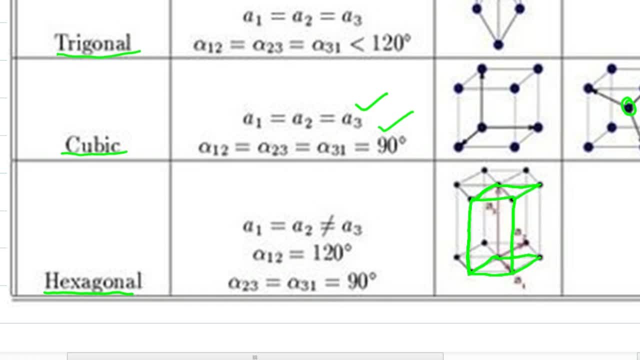 This specific formation is for the hexagonal. We have decide A1, A2.. It is the side A1 and A2.. And this is your angle. that is 120 degree, And these two are the 90 degree angles. So now we come to the bases. 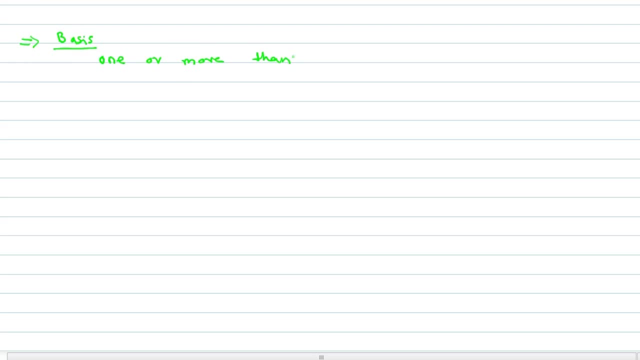 So what are bases? So we have 1R, more than 1.. Atom or ions that are assigned to the lattice points in crystal structure are called bases. So let's suppose these are the lattice points. We have four lattice points. 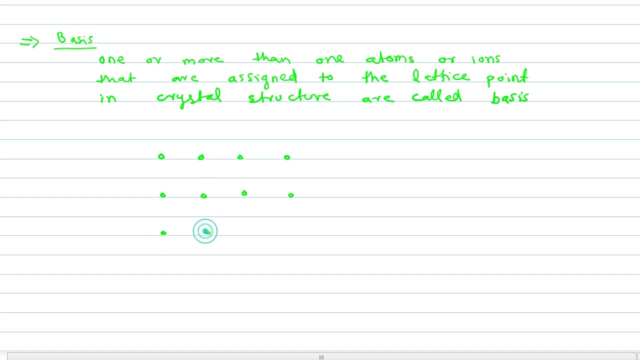 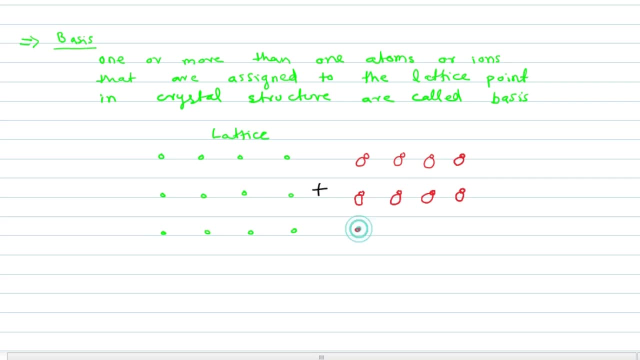 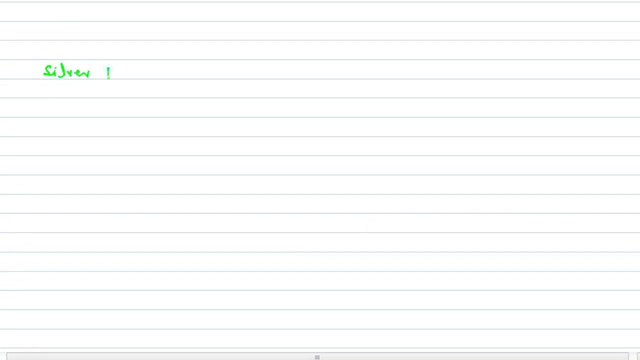 So if we assign these molecules to these specific lattices, so combination of these two, And let's suppose which one of them, will give us a crystal structure. So to understand this, we take two different examples. So first one is the silver. 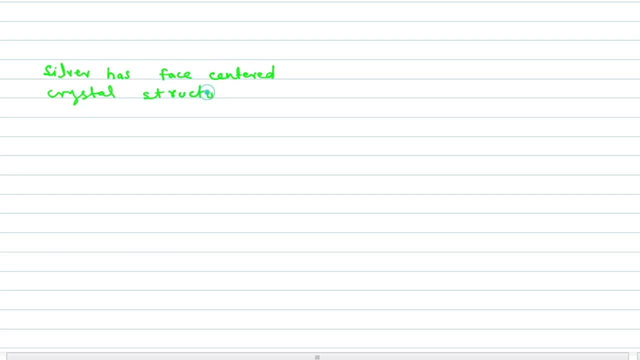 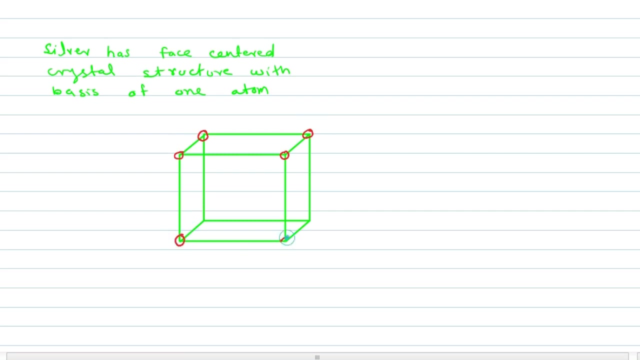 So silver has a phase centered crystal structure with the bases of one atom. So this is a cubic structure, all the atoms according to the face center. cubic structure. we have one atom at the each corner and one atom at the each face. So number of corner atoms is equal to 8 and their contribution 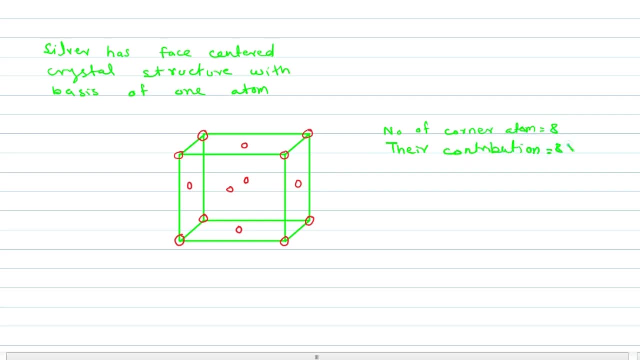 to the unit cell is equal to 8 multiplied by 1 over 8.. We multiply by 1 over 8 because one atom at the corner is contributed by 8 unit cells, So its total contribution is equal to 1.. Similarly, 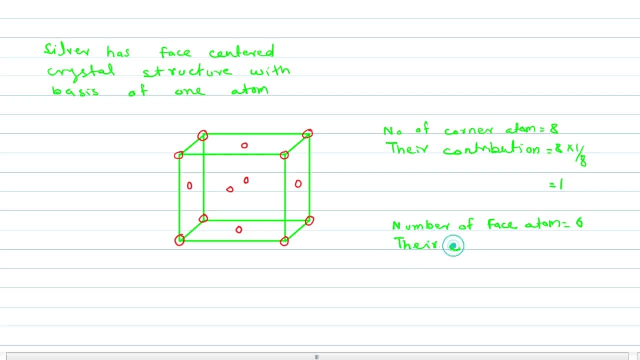 number of atoms at the face are 6.. So their contribution is equal to 6 multiplied by 1 over 2, as face atom is contributed by 2 unit cells. So total number of atoms here are 3 plus 1, that is. 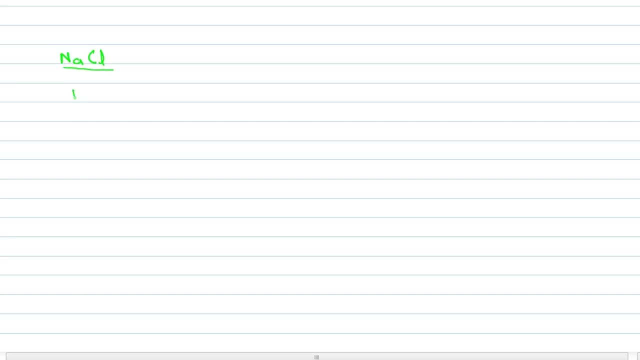 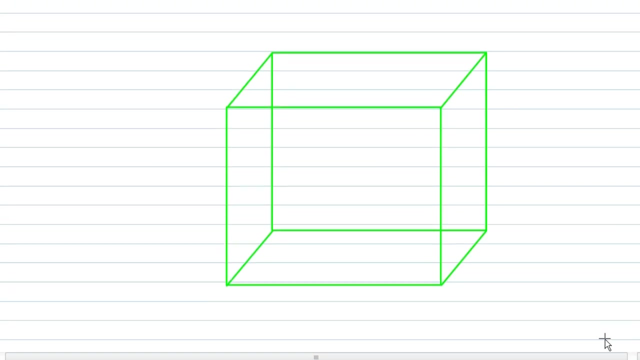 equal to 4.. Now we take the example of the NaCl, that is, sodium chloride. So for sodium chloride, that is a face centered cubic structure with basis of NaCl molecule, or we can say it has basis of two ions that are Na plus and Cl minus. So this is a cubic structure. Now 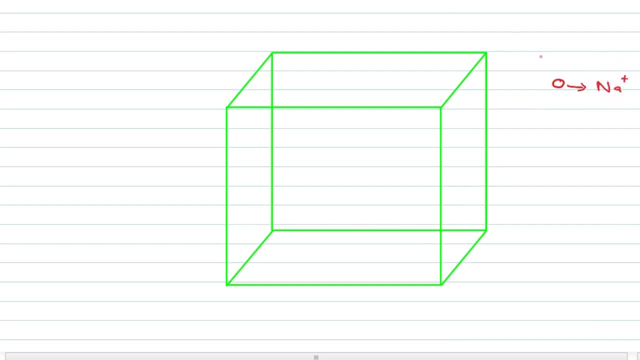 we place atom. So if this red circle show the sodium ion, So we place it at the FCC positions, So we can say its basis is at the f of 1. So this is go somewhere between 0 and 0. 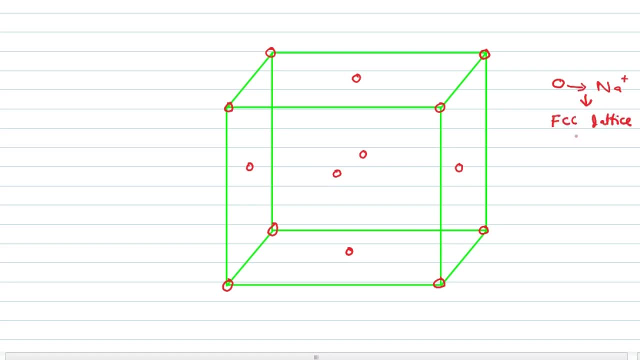 So we take patient the same value with respect to the NaCl molecule. So if the patients have at one also will have the same amount of NaCl molecule being the same as their multi sample and filling here and there. also 50 かm per liter. 채. Altering by: i catahontos from a 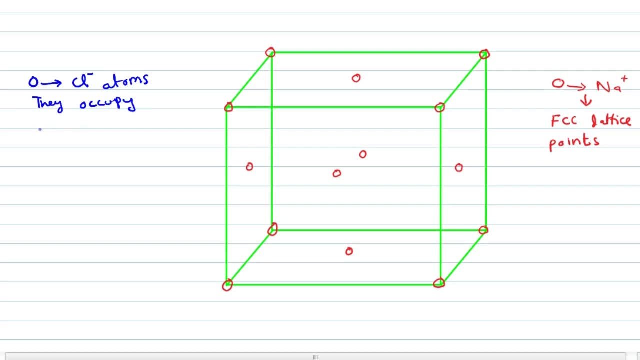 single phase. so this is for ВCL. I plusところ there, which is the Zeol state. So what is a Mesh Ca a? They occupy the octahedral position in FCC, If you do not know about the octahedral position, so I have made a separate video on this. 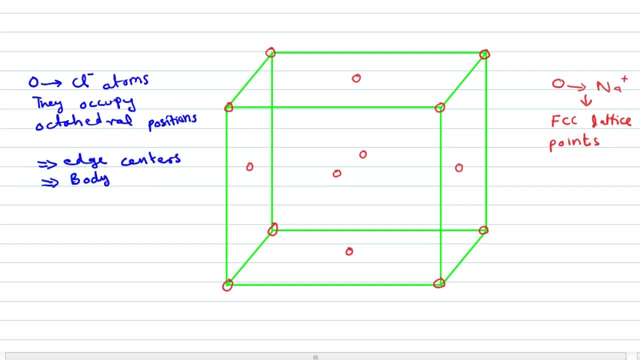 I will put link in the description. So octahedral position are present at the edge centers and body center. So we put one chlorine ion at the edge center. So the position of the sodium ion and chlorine ion are totally interchangeable. You can interchange them. 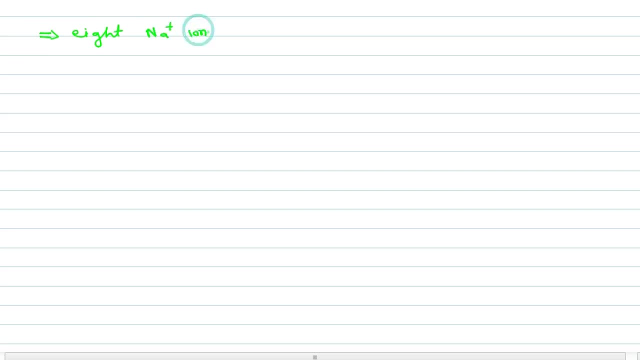 So now we calculate the basis for this one. So we have 8 Na plus ions occupy corners. So their contribution to unit cell is equal to 8 multiplied by 1 over 8, that is equal to 1.. Okay, Similarly, we have 6 Na plus ions that occupy faces.